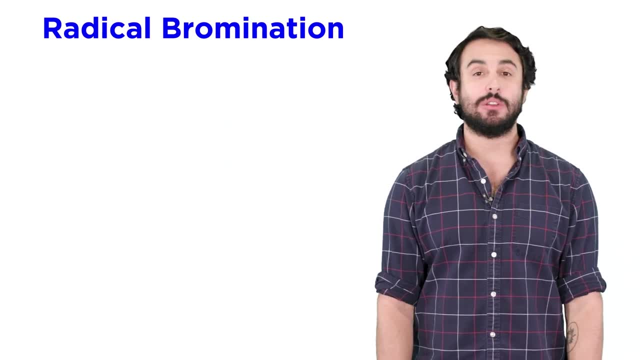 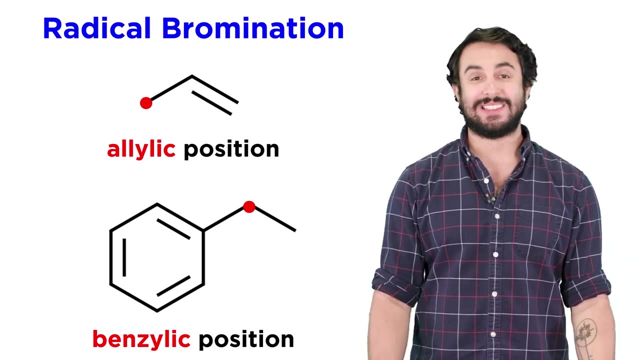 There is another context in which we can brominate at a particular location on a molecule other than an alkane. This can be referred to as bromination at the allylic or benzylic position. Let's take a look at what these positions are, how the reaction works and precisely. 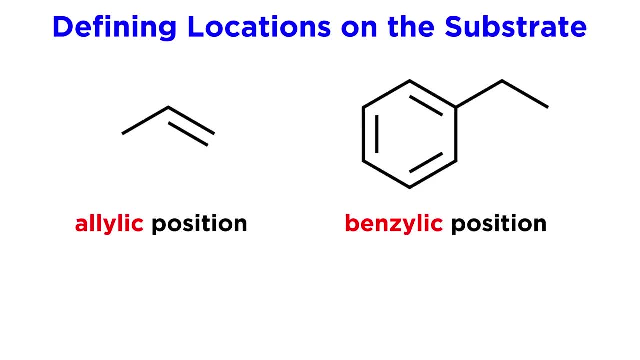 what type of reagent will promote this reaction? First, let's clarify what we mean by the allylic or benzylic position. When we say allylic position, we are referring to the carbon adjacent to a double bond. So, given this alkene, this would be the allylic position. 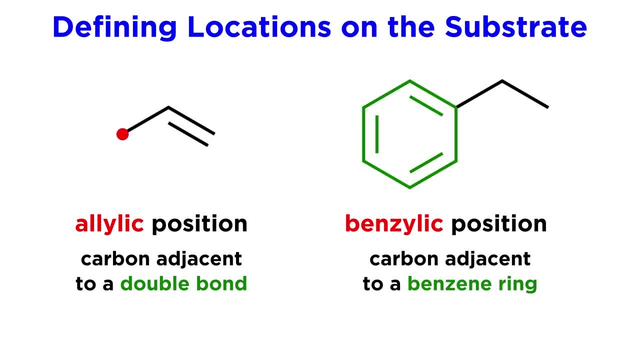 When we say benzylic position, we are referring to the carbon adjacent to a double bond. So, given this alkene, this would be the allylic position. When we say allylic position, we are referring to the carbon adjacent to a benzene ring. 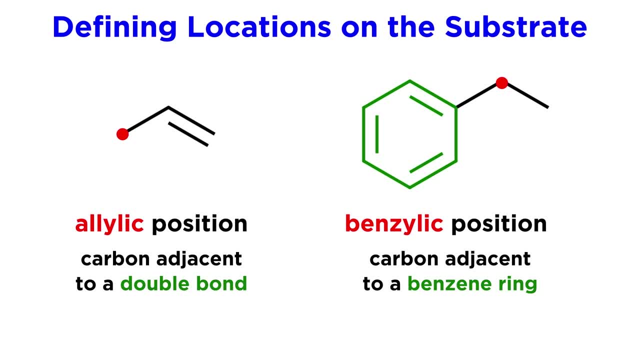 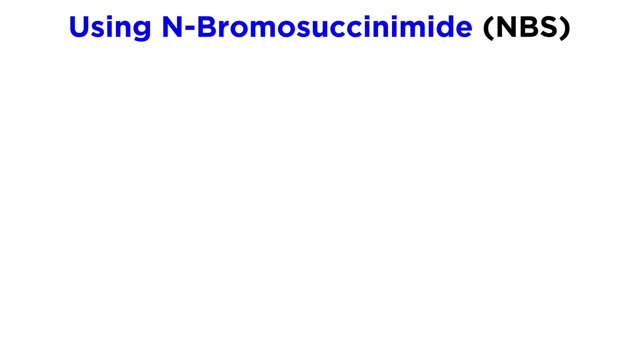 So, given this molecule here, this would be the benzylic position. The kind of bromination we will be performing will involve placing a bromine atom specifically at these locations. The reagent we will be using to achieve this is called N-bromosuccinamide, or NBS for short. 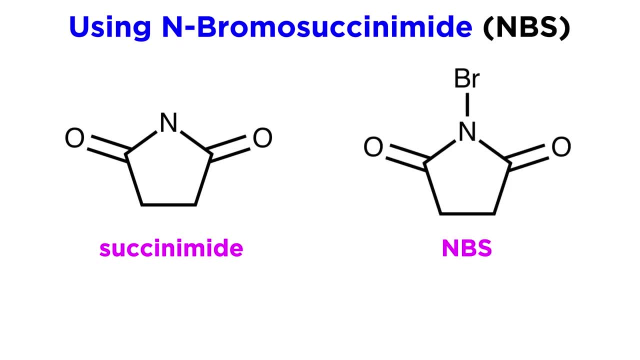 Structurally speaking, succinamide will be a bromine atom. Structurally speaking, succinamide will be a bromine atom. Structurally speaking, succinamide will be a bromine atom. N-bromo looks like this and N-bromo refers to the presence of a bromo group on the nitrogen. 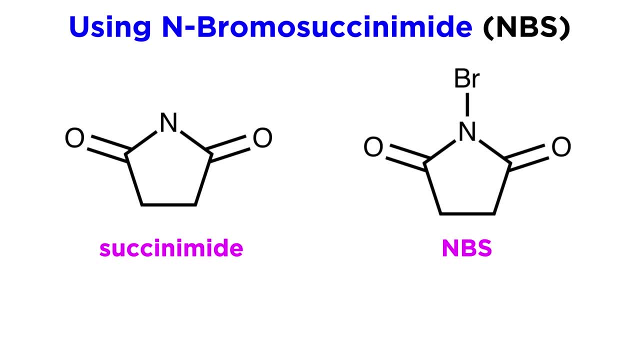 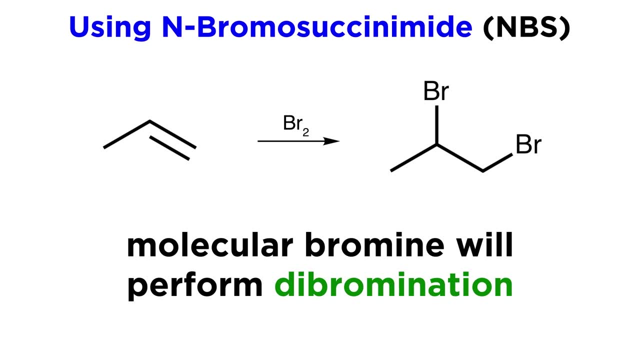 atom. so this is N-bromosuccinamide. The reason that we would use this reagent rather than molecular bromine is that, if we are trying to brominate a molecule with one or more pi bonds, molecular bromine tends to do dibromination with pi bonds, something that is not of concern when the substrate 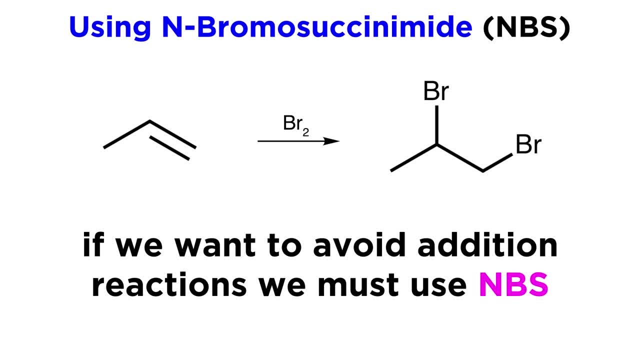 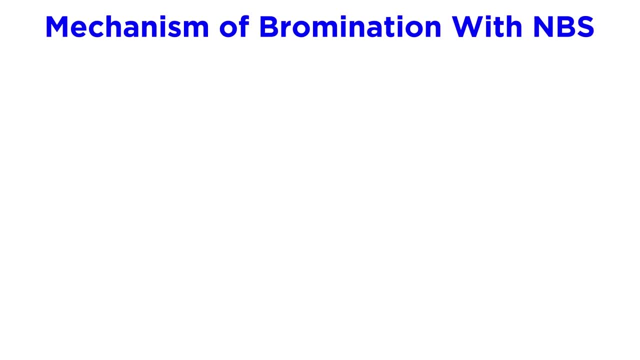 is an alkane. If addition reactions are to be avoided, we will want to use another reagent, and that will be NBS. The mechanism works as follows: In the presence of hydrobromic acid catalyst, small amounts of molecular bromine will be. 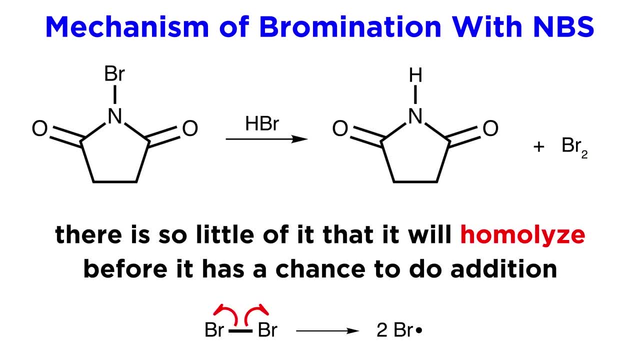 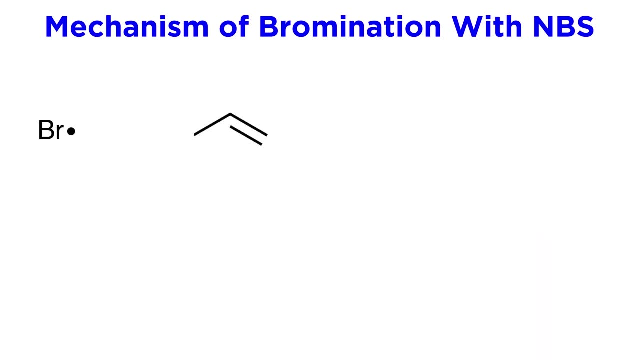 produced. This will be in small enough amounts that there is enough time for bromine to undergo homolysis before having a chance to interact with a pi bond, so there will be bromine radicals in solution. Now let's allow this to interact with an allylic substrate.